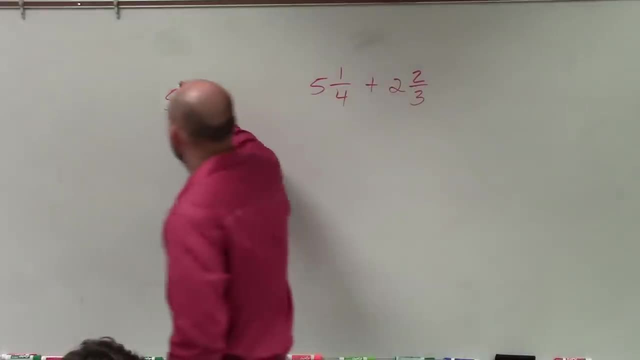 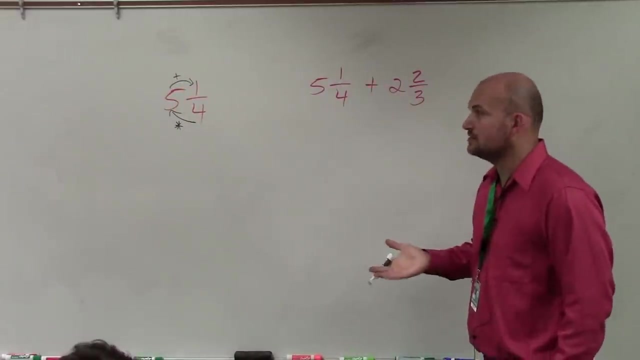 So 4 times 5 is 20.. Then you're going to add that sum or that product to your numerator, And when you do that you're still going to leave it over 4.. So 4 times 5 is 20, plus 1 is 21, over 4.. 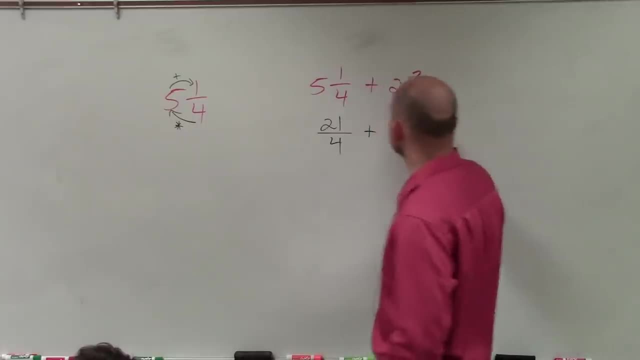 Then I do the same thing over here. so that's 21 over 4.. Plus 3 times 2,, which is 6, plus 2 is 8.. So now I've written it as improper fractions and now I have 21 over 4, plus 8 thirds. 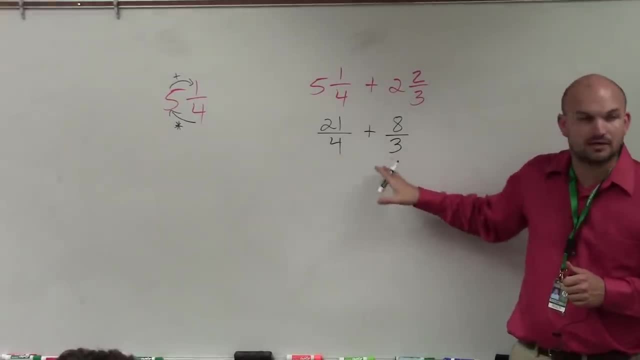 However, what we notice here is we have two uncommon denominators. right, They're not like denominators. So, Stephen, what we'd want to do in this case is we want to compute the least common denominator, That means, the smallest number that both 4 and 3 divide into. 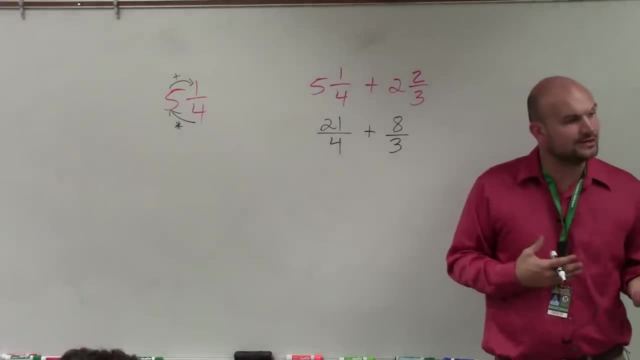 So to do that, What we need to do is one easy way to do that- is just to multiply your denominators 4 and 3.. That's going to give you 12.. We both know that 12 is divisible by 4 and divisible by 3, right. 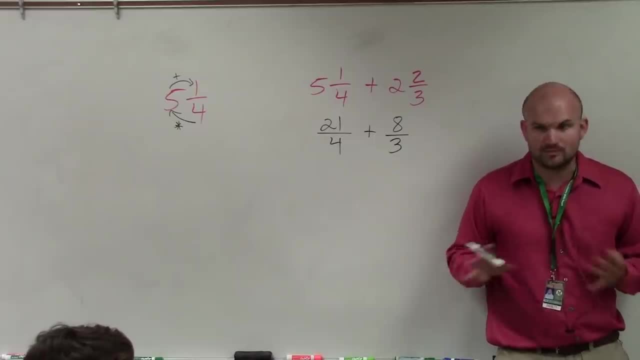 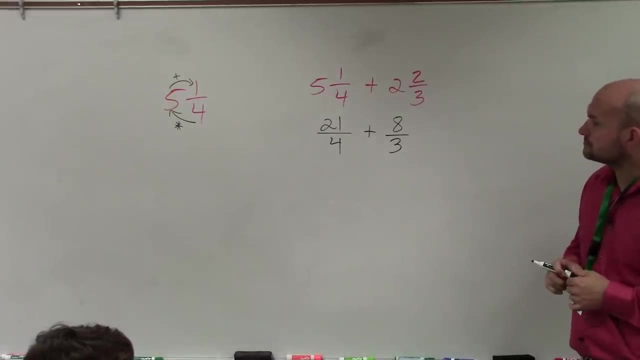 However, the next example I'll do. you'll notice that not always just multiplying denominators is the best or fastest or easiest way to determine the least common denominator, But we'll do that next. So in this case I need to multiply both of my denominators to get them to be 12.. 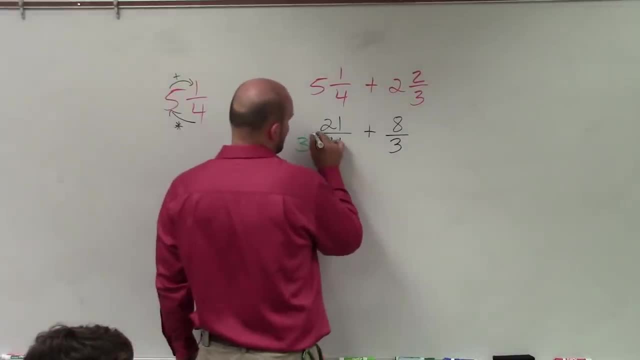 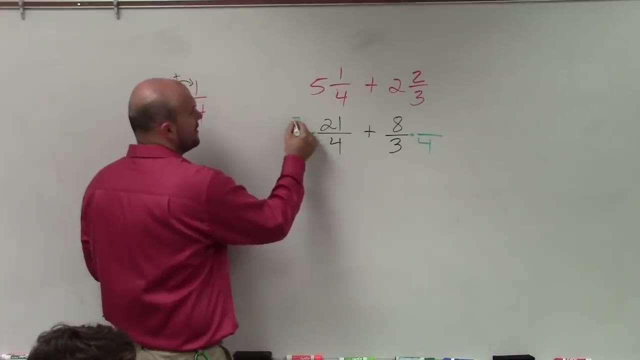 So I'm going to multiply this. I'm going to multiply this denominator by 3, and this one by 4.. But it's very important, ladies and gentlemen, when you're multiplying to produce a common denominator, that you multiply the denominator and the numerator by the same number. 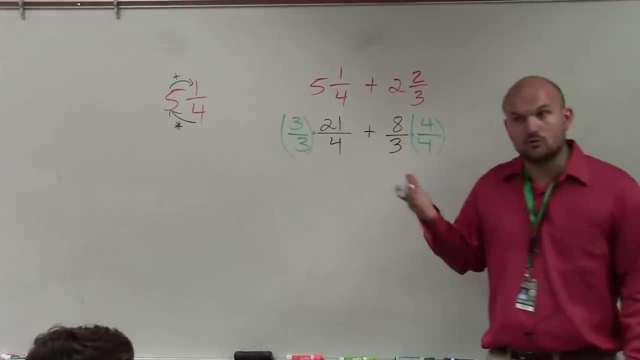 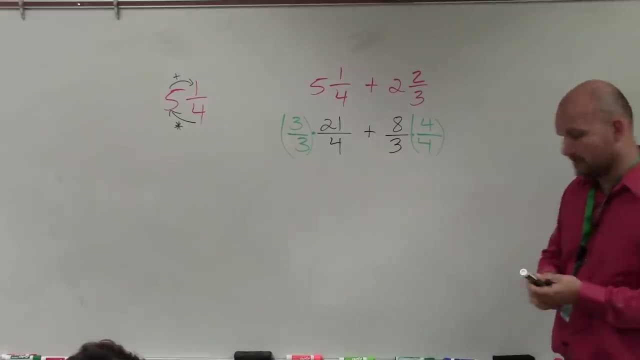 The reason being is we want to produce what we call equivalent fractions, Fractions that have the same value but are in different form. For instance, 3 over 6 is equivalent to 1. half right, They're equivalent fractions. So now I'm going to need to multiply. 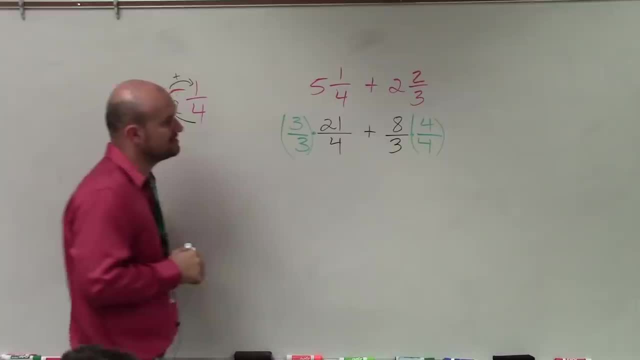 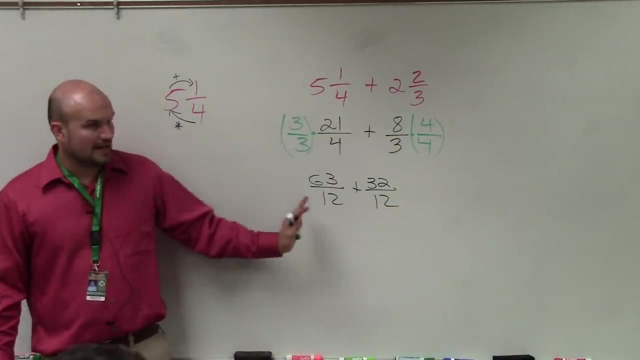 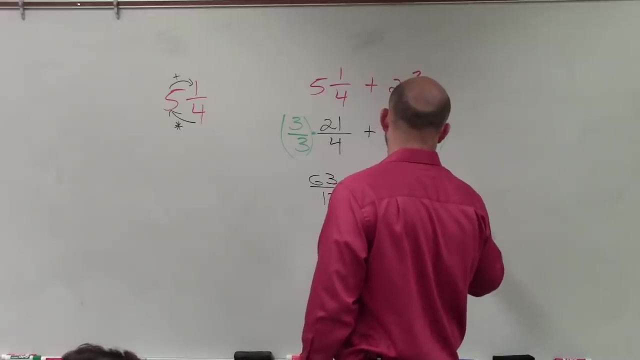 So when we multiply, we just multiply the numerator times the numerator denominator times the denominator 3 times 21 is 63 over 12, plus 8 times 4 is 32 over 12.. Now I have common denominators and I can add my numerators, which would be 95 over 12..